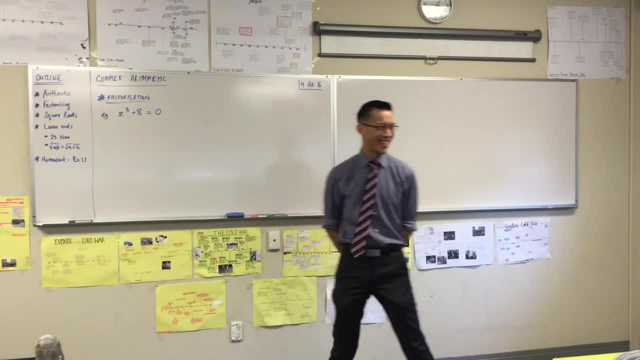 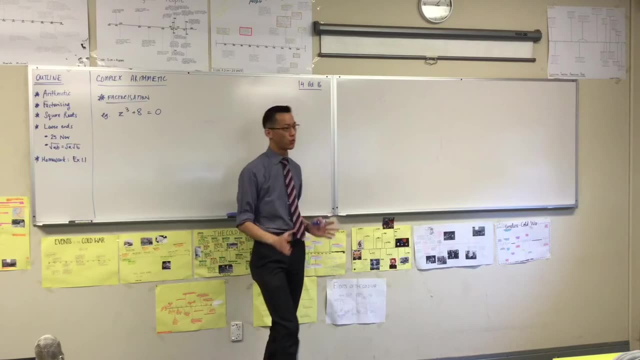 This kind of looks a bit like year 7, then year 8, then year 9.. Now that you know what this mathematical universe is really made of, it's like you have to rewrite all the rules, and it's kind of cool. So factorization. 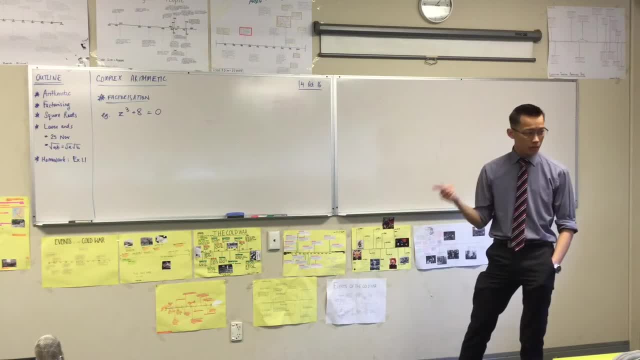 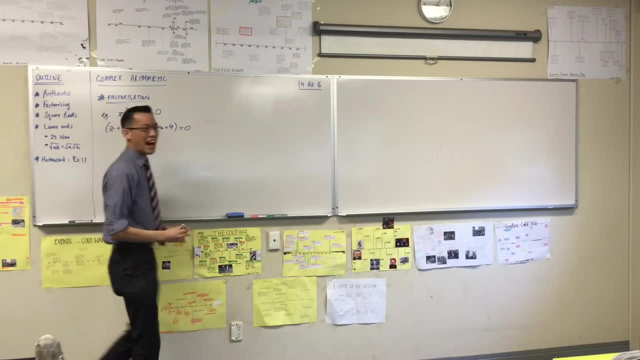 let u plus 8.. Now, as two-unit students, you can do something with this. Complex numbers completely aside, how would you factorize this thing? Okay, good, Now I will point out: you guys are part of that wonderful generation that has a reference sheet. 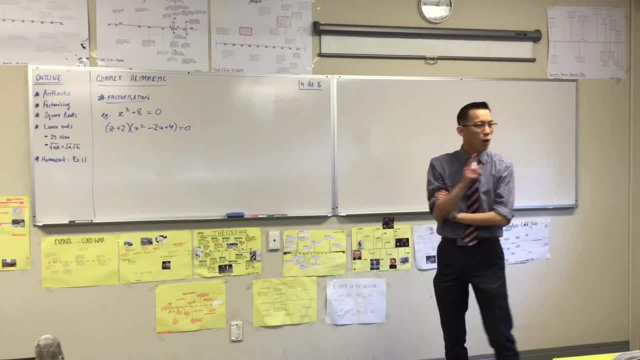 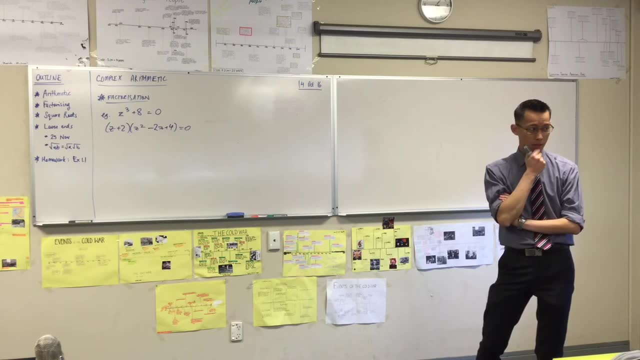 I didn't have a reference sheet, so I had to memorize this kind of thing. I will point out, though, the reference sheet- honestly the two-unit side at least- is not for you guys. You guys should all be able to have what I had, which is all of these kinds of results, up here, because the reference sheet 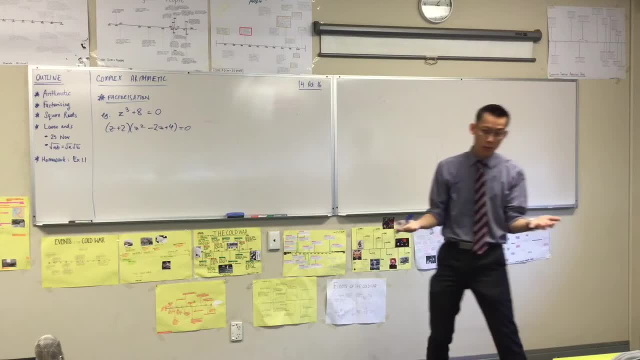 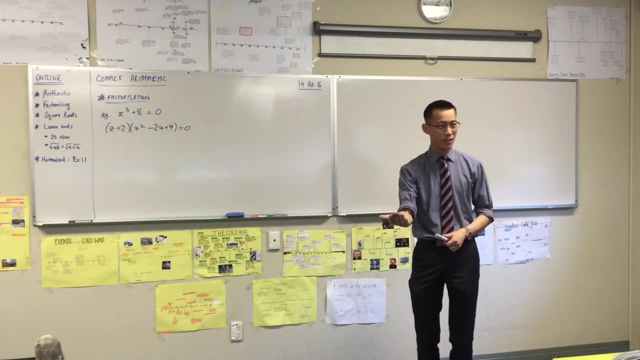 is there to help you. okay, But, as you can imagine and as you may have already discovered in the assessments you've had with a reference sheet, the reference sheet comes with a time penalty. right, You use it. you're looking for something, not just saying I know this and then you put it down on the page. okay, 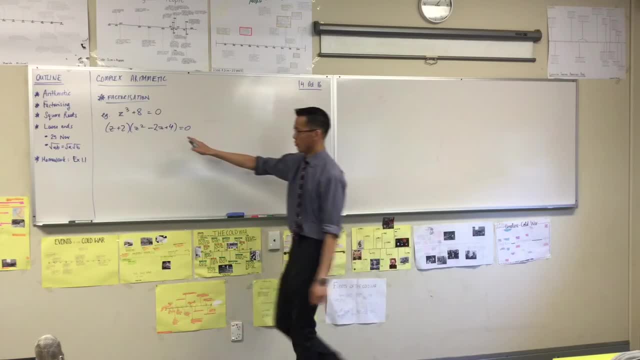 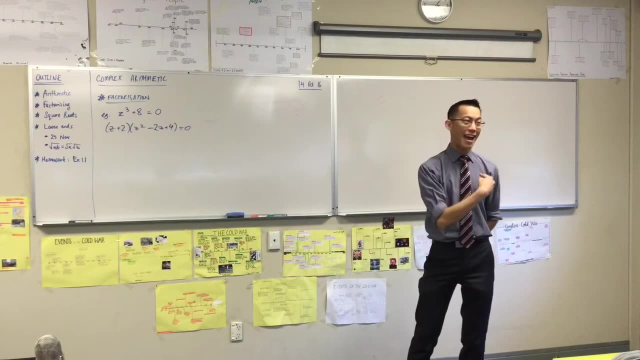 The extension one stuff. that's a different ballgame, but you guys should all be able to do this like without thinking: okay, It also helps you not to have to look to something to check it When I had to remember it. 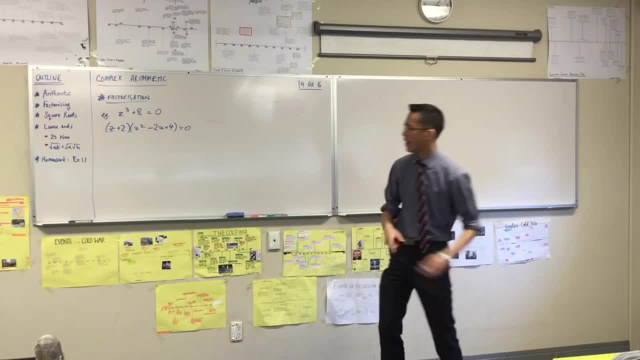 I had a mnemonic for this. You guys know what mnemonics are. right, My mnemonic for this was soap, Because of course, the hard part, as we just noticed, is the signs Everyone else gets, like the squares and the twos and that kind of thing. 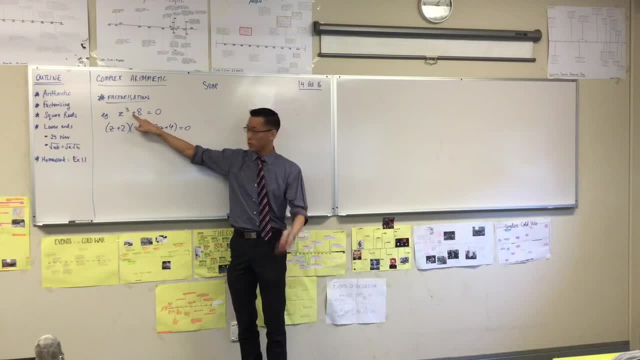 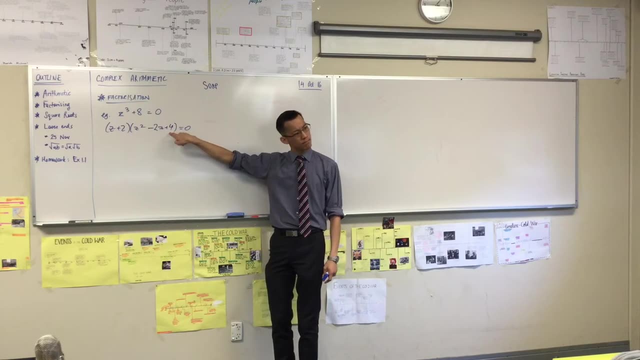 So the signs go like this: This is a plus, right, It's the sum of cubes. So the signs that you get, there's three of them. they always go like this: Same opposite, always positive. Did you notice that If I did z cube minus a, if I did the difference of cubes, this would be the same minus. 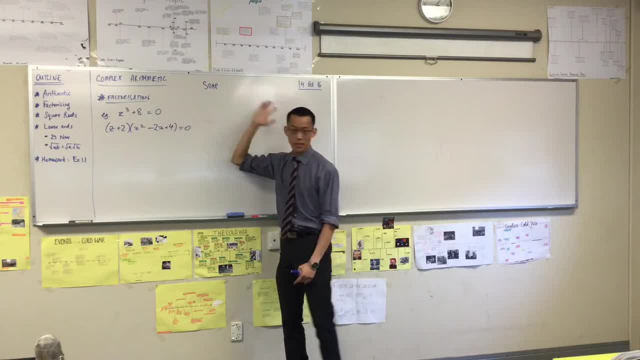 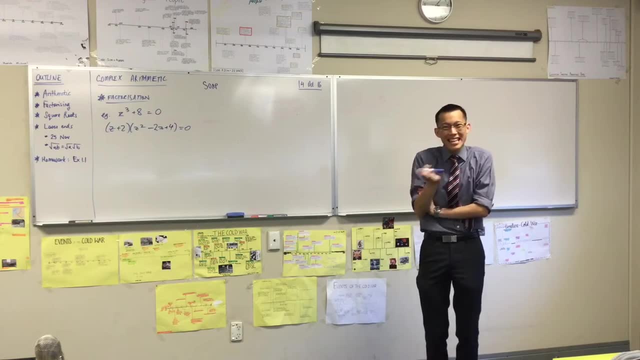 opposite plus- and this guy's always a plus- okay, Anyhow, if that's useful to you Now as a two-year student, or even an extension one student, you would go home at this point. okay, It's done, It is factorized. There's nothing more to do with this question. One mark, right. 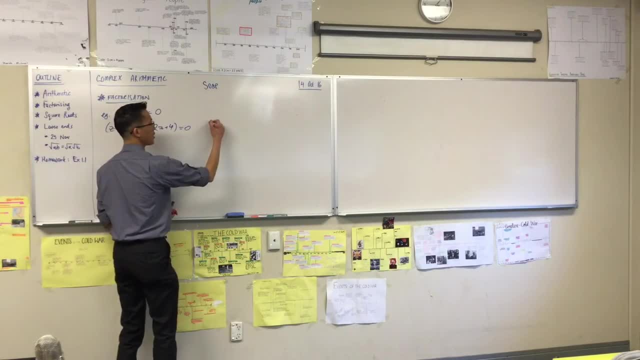 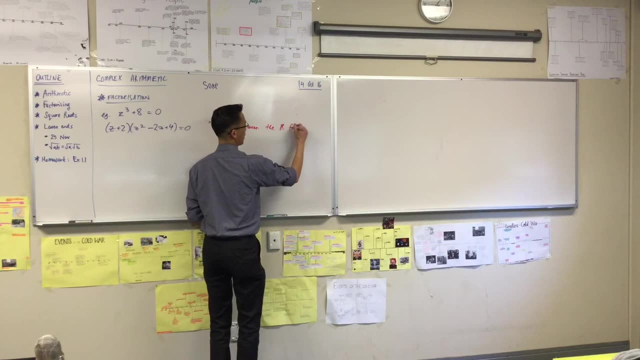 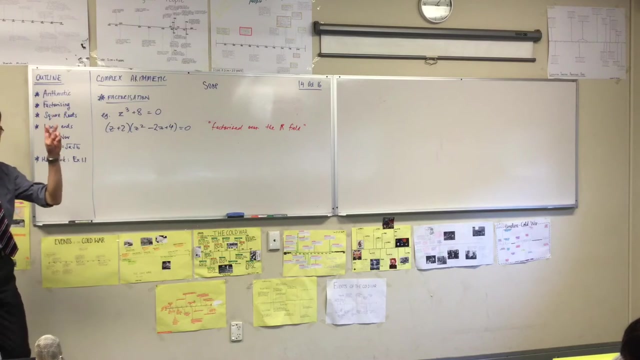 What you've done. you might like to put this, write this over on the side here: What you've done is you have factorized this over. There's a couple of different ways to say this. You could say it's factorized over the set of real numbers, or you could say it's factorized over the real number field. okay, 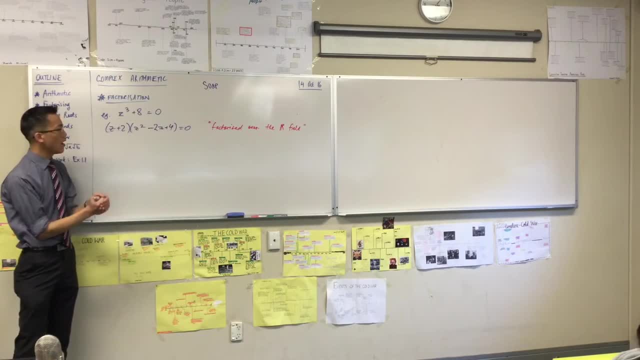 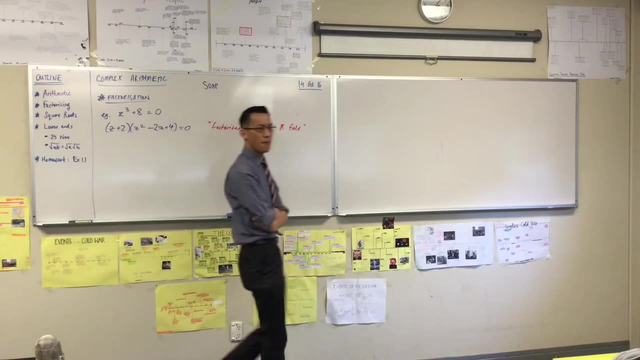 Which is just a fancy flowery language name for the set of real numbers. but we can go further now. okay, We know that this guy over here, we can deal with this. no matter how messy it is, we can deal with it, because complex numbers allow us to factorize anything. okay. 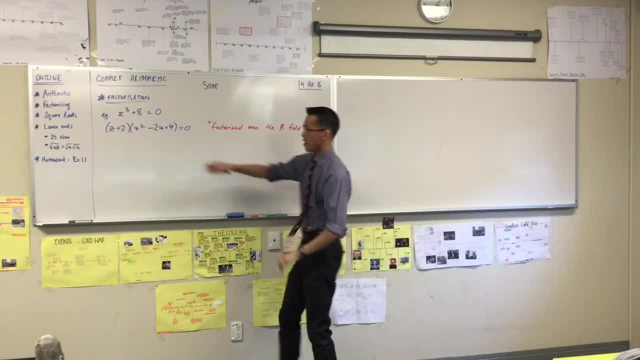 Now you can do one of two things here. Have a look at this. You know I can't think of a nice pair of numbers that's going to add to negative 2 and multiply to 4, right? So when you get presented with a quadratic, 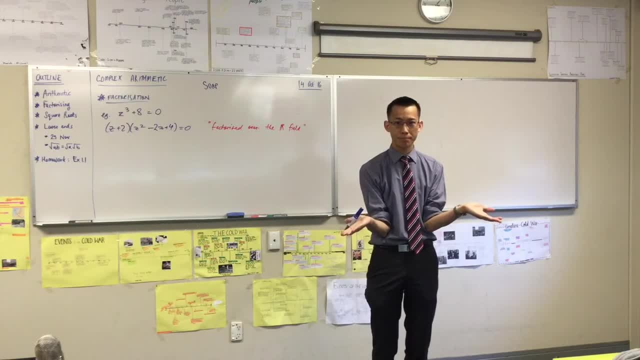 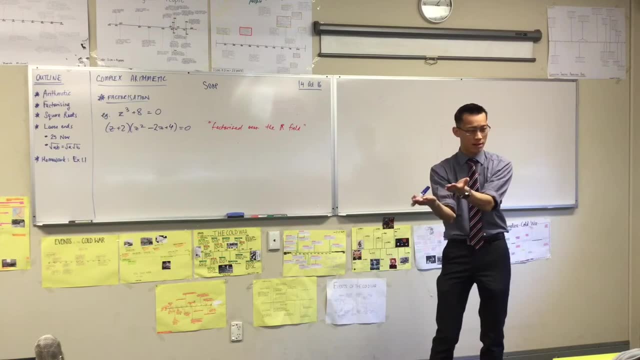 that you can't factorize. neatly, what are the two options you've got? You can either go to the formula right, And then you get two roots out and then you use the roots to factorize, or alternatively, you can complete the square. okay, Now honest question: which would you prefer to do? 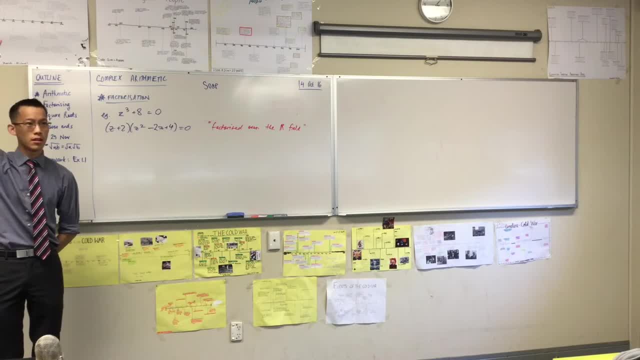 Complete the square. Who would go for the quadratic formula? just out of curiosity? Okay, yeah, cool. Now I'm just going to tell you right now: when I was in year 11, I would have probably gone to the quadratic formula. That was just what I was more comfortable with. 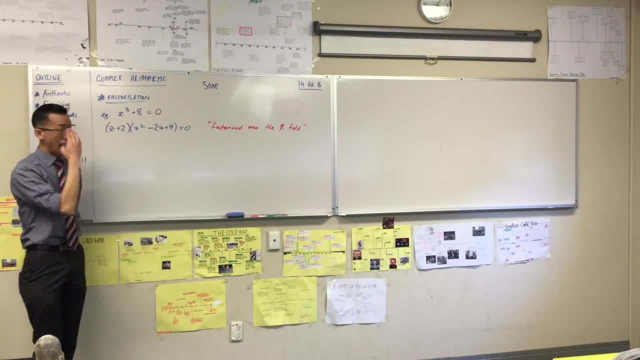 but completing the square always weeded me out a little bit and I always had problems with it. okay, However, I'm going to suggest like now, as a teacher, I've kind of gone the other way and I'll tell you why. Number one, you can't get away from completing the square. 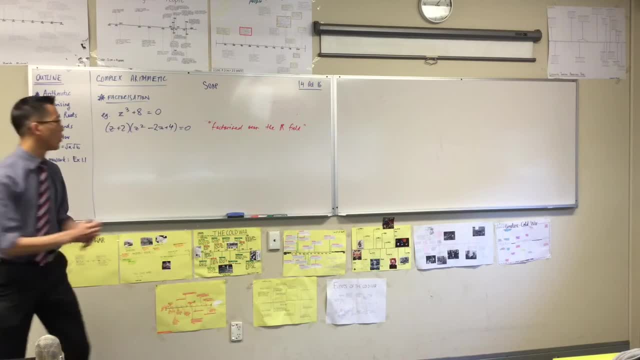 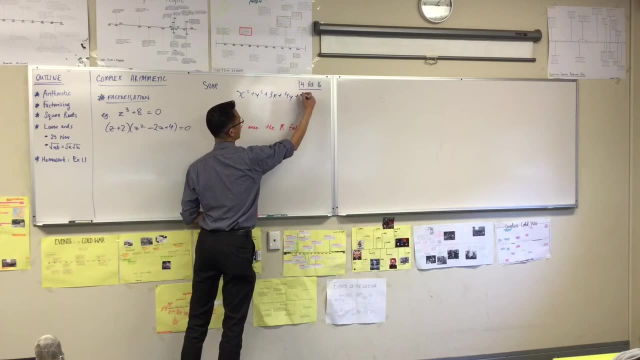 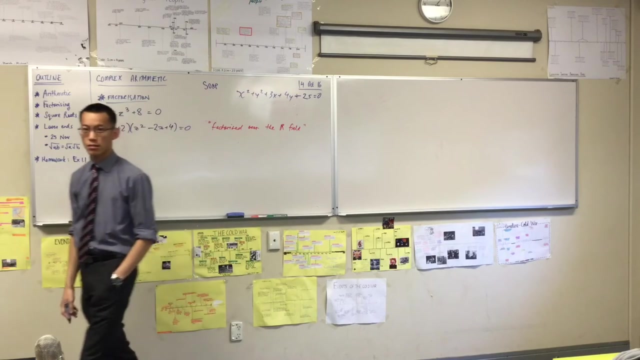 Like. you can't avoid it As two unit students. even if you want to work out where on earth the center, you want to work out where the center of that thing is right, You're gonna have to complete the square. the square. you can have to do it twice, okay, so you can't avoid this skill, it's. 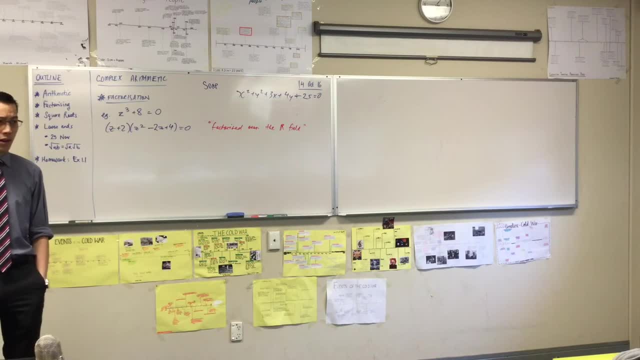 a bit like graphing. I know some people don't like graphing because like, oh, it takes me forever. you can't get away from graphing, you might as well master it. okay, kind of the same deal here, so let's all together complete the square on this. 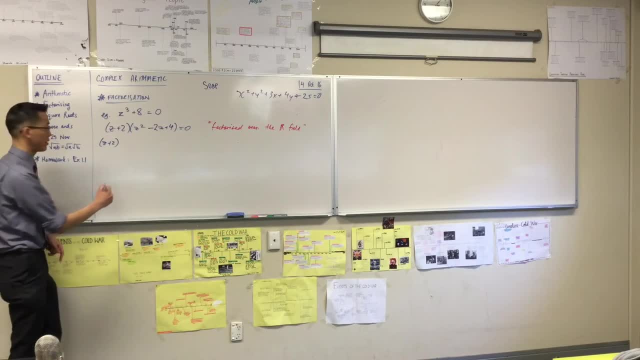 guy. right, you've got your Z plus two out the front there, happily. see you now. here's my Zed terms. what do I do to complete the square? is that right? it is right, because the way you complete the square is: you have this coefficient, then you square it okay. so plus one is fine. that leaves a plus three over here. yes. 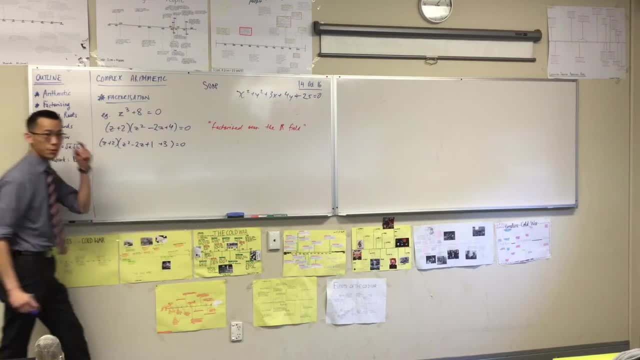 like, because that's the four that we had before, so that's equal to zero. okay, now, the reason we added this one, or we took out the one, rather, is so that now I can say this part here can be rewritten as what Zed minus one squared. okay, now, before I, 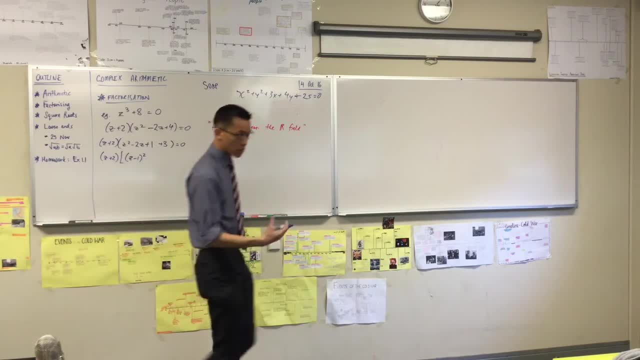 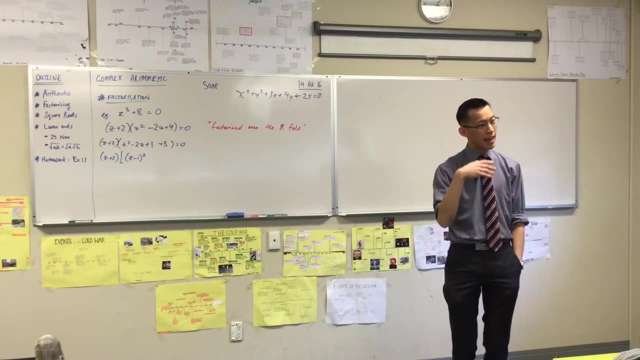 write the next bit right? the whole point of doing this is so I can factorize a little more right. but something squared plus something squared is no use to me, or something plus something. but if I can have a difference I can factorize that right if I have a difference of squares. so I'm going to rewrite this guy over. 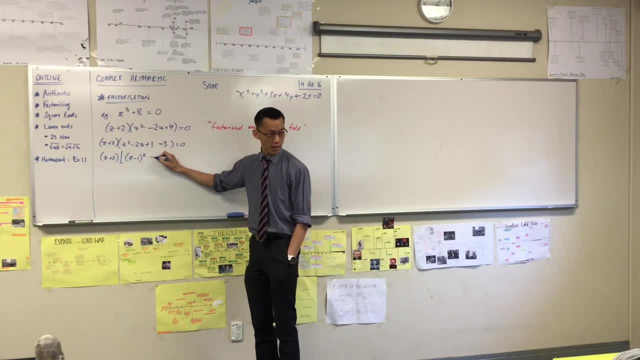 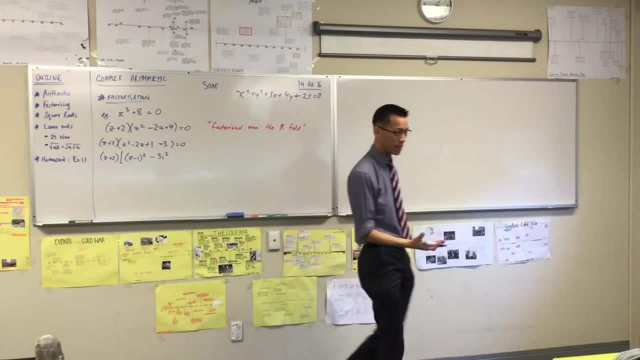 here I'm going to rewrite it as not plus but minus. and, of course, if I take this one over here, I'm going to rewrite it as not plus but minus. and, of course, if I take a negative out, well, I better put a negative in. see what, what I did there. 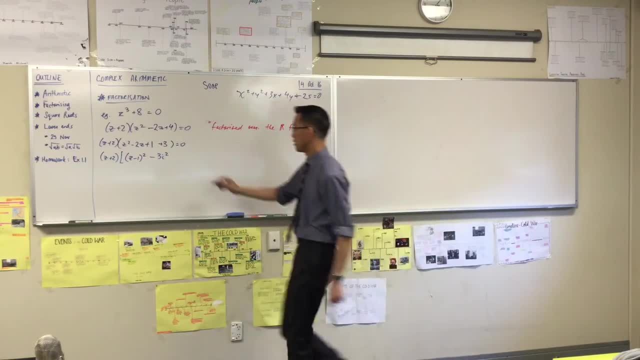 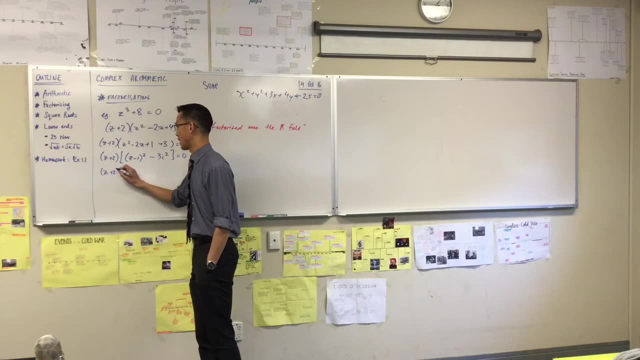 right. so complex numbers allow us to muck with this a little more, because now I can factorize it further. yes, okay, let's have a go at this. the Z plus two is still hanging out the front there, patiently waiting for us to get on with the rest of it. okay, what's going to happen here? actually, I should have drawn. 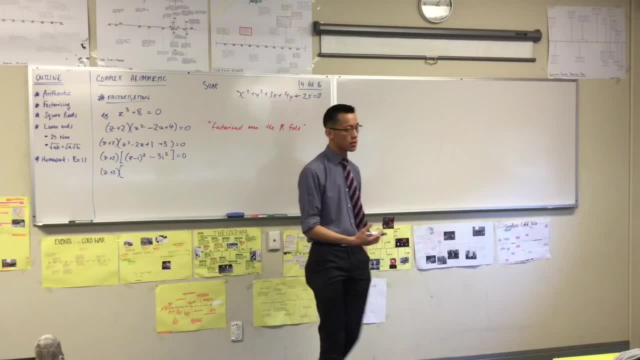 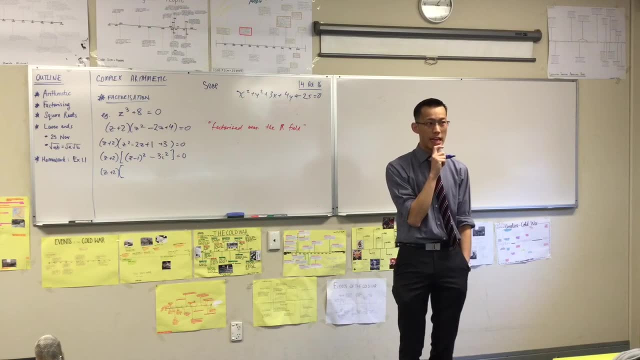 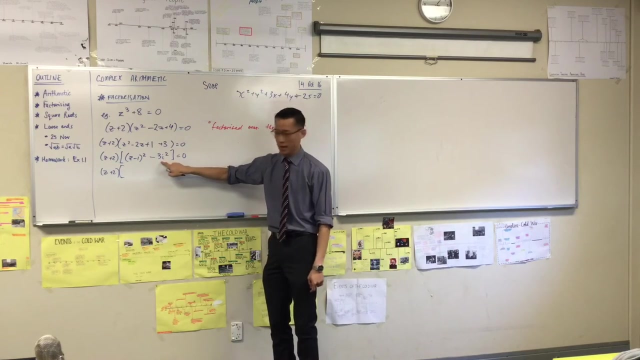 a square bracket. what's going to happen here? I can do difference of squares. what's A, Z plus one. what's B- careful, it's root three. I do you agree with that? like, if I square root three, I that'll give me this, okay. so I'm going to do this is a squared minus B squared. 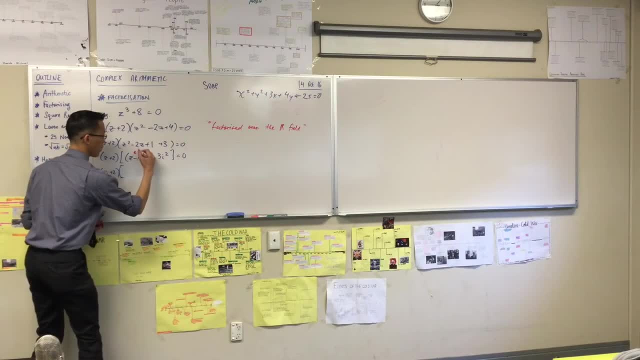 in fact, you may even like to write that this is a squared minus B squared. so what I need on the next line is a minus B, a plus B, and you just identified for me what a and B are. so it looks like this: I think there's a. 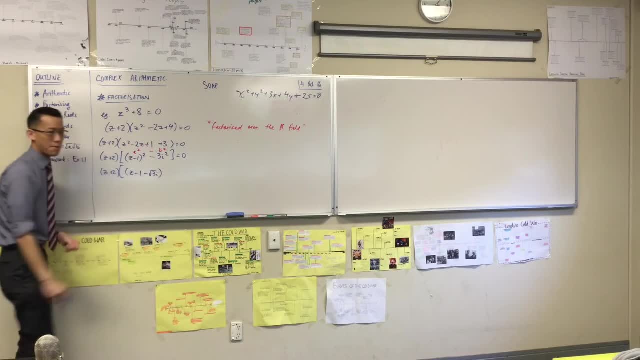 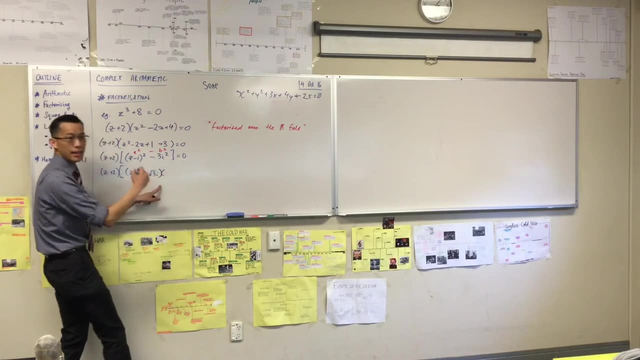 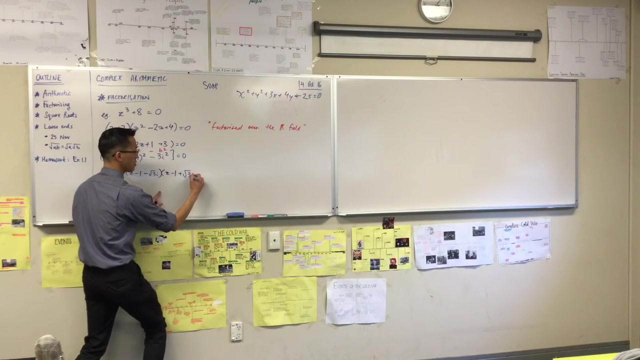 there is a minus B. are you happy with that? see what I did. okay, careful. there's the a minus B. now I need the a plus B. okay, that's gonna look like this: a is still the same, but this is plus B. okay, are you feeling like an extension? two: 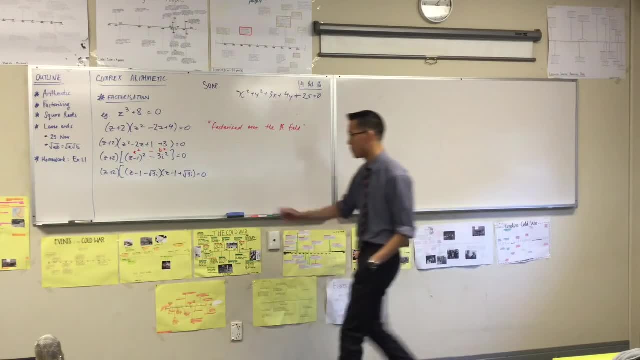 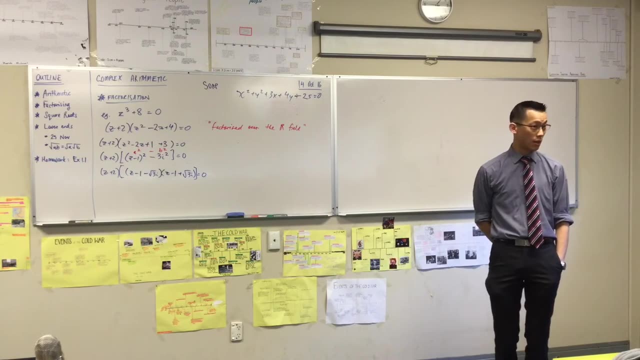 student: yeah, okay, so this is. this is hard to wrap your head around and make sure that you accurately do your numbers. okay, but that's it. in fact, I don't really need either this square bracket. I'm done now. this is not factorized over the real field. we had to appeal to a new kind of number to get to. 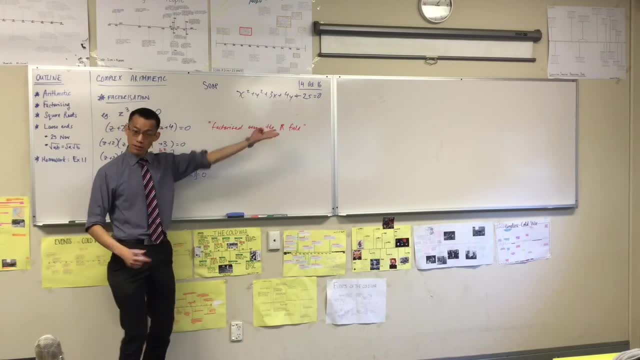 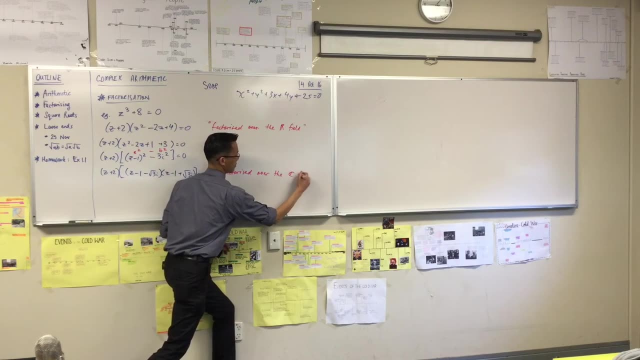 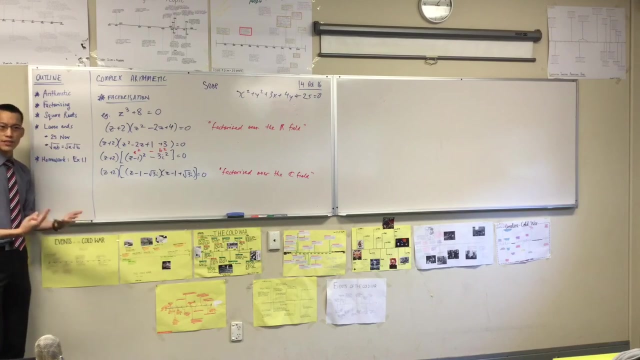 this point, okay. so therefore, instead of saying, factorize this over the real field, you have surprise, surprise, factorize this over the complex field. now, not only have you done that, but I want you to notice there's a qualitative difference, not just the fact that we've used different numbers, but there's a 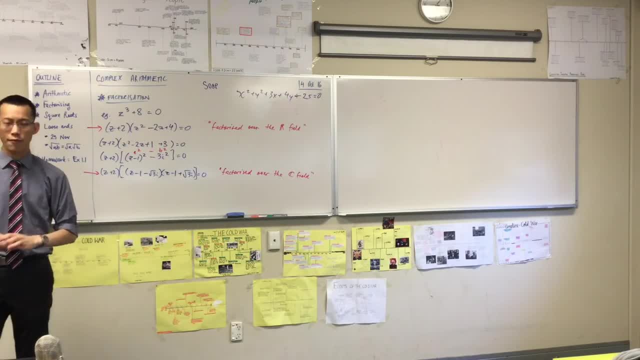 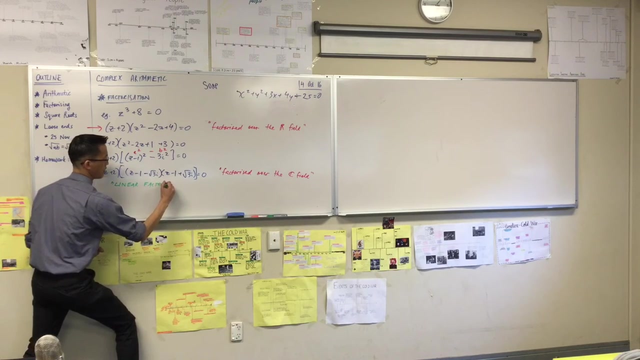 qualitative difference between this line and this line, and the last line is better for a very important reason. this is what we call. in fact, this is worth writing down to in another color, got it? this final white here is called the linear factorization of the polynomial. I started with the linear. 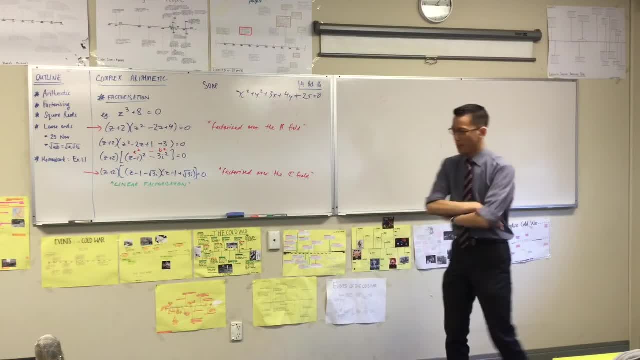 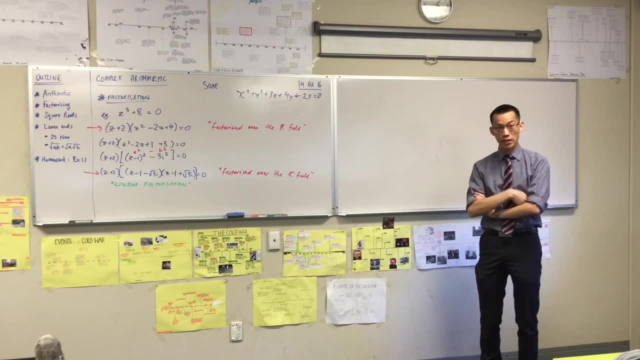 factorization- now I'm a bit obsessive names. anyone who's been in my class before knows that. why is it called the linear factorization as opposed to the linear factorization? as opposed to linear factorization, It goes to earlier factorization I found. 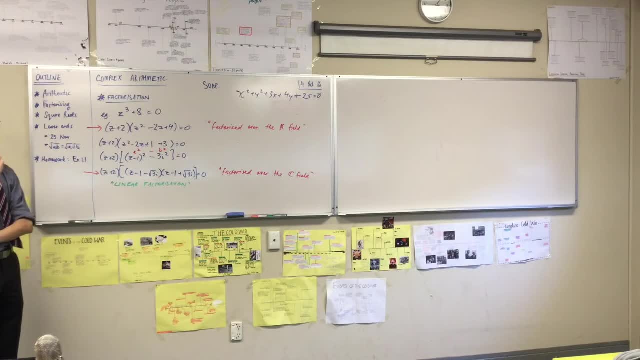 Factorization- yeah, Suggestion, Because it can be graphed. I can graph this right. I can grammar this. Importantly, when I graph it, have a look at these factors right. Like factorization is, can you break something up into its pieces? okay, 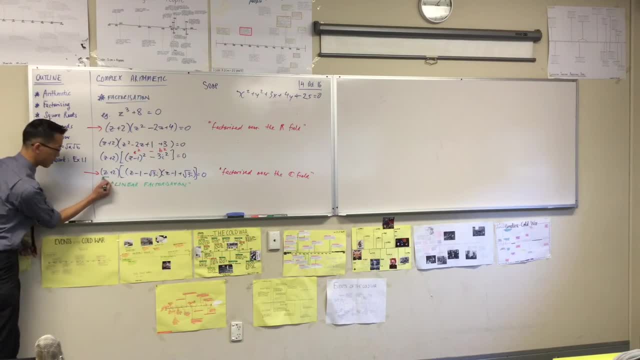 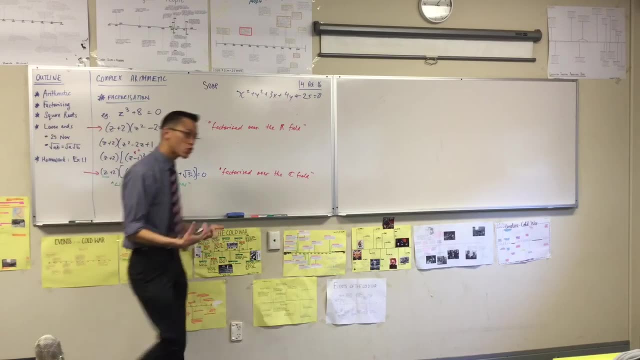 All of the factors are. look at the powers of the factors. do you notice? There's a z to the power of 1, then there's another z to the power of 1, and then you get another. They're all straight lines, okay. 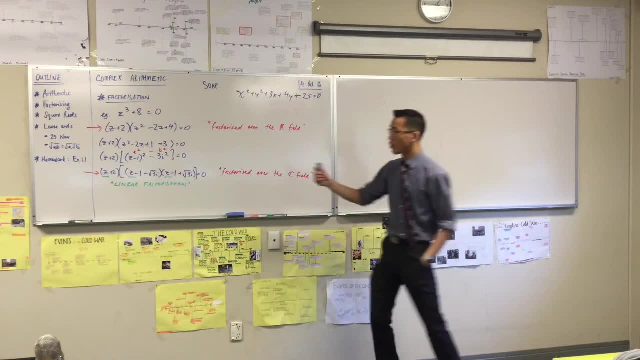 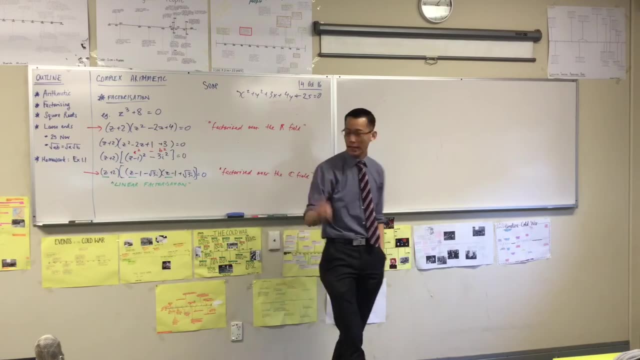 As opposed to go look at that real factorization I had before. You got one of them. one of them is a straight line, but the other one is a parabola, right? So that's not a linear factorization, okay. 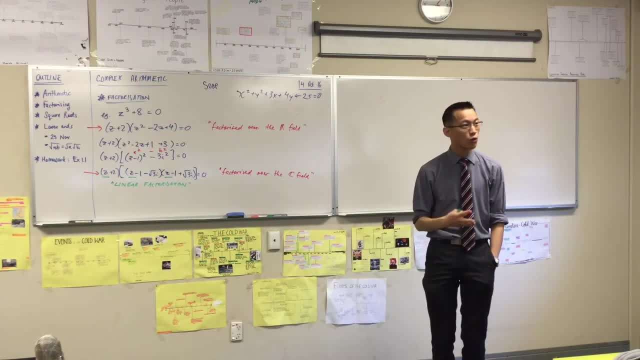 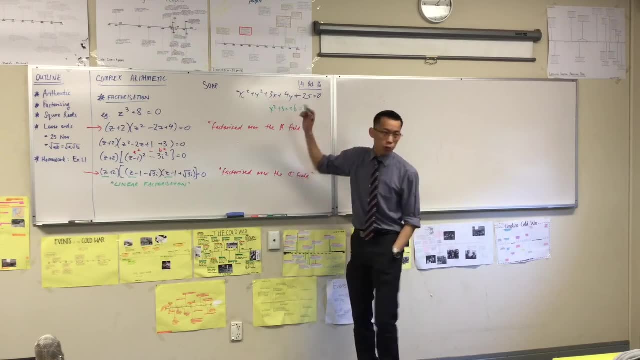 Now, linear factorizations are awesome because they tell you solutions. right, That's the whole point of when I give you something like x squared plus 5x plus 6, right, The whole reason we obsess over. can you factorize that and be really quick and accurate at it? 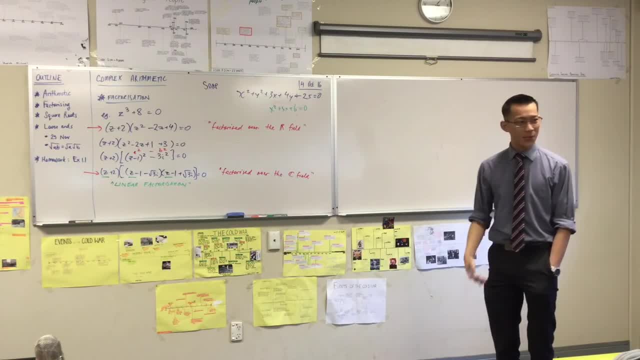 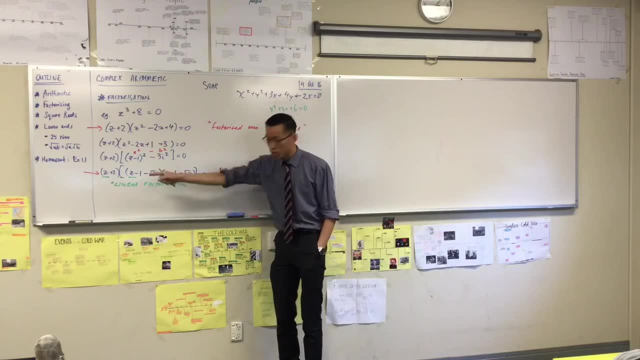 is so you can give me the solution. You can give me the solutions very quickly, okay? So now, even though it wasn't the point of the question, I just wanted to factorize, you can all tell me what the solutions to this are, right. 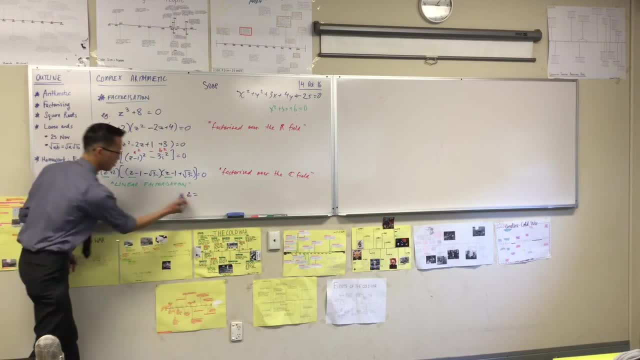 Can you tell me z equals? there's one easy solution, the first one right, which is 1 minus 2, okay, By the way, negative 2, minus is an operation. negative is an adjective. Negative 2, that's fine. 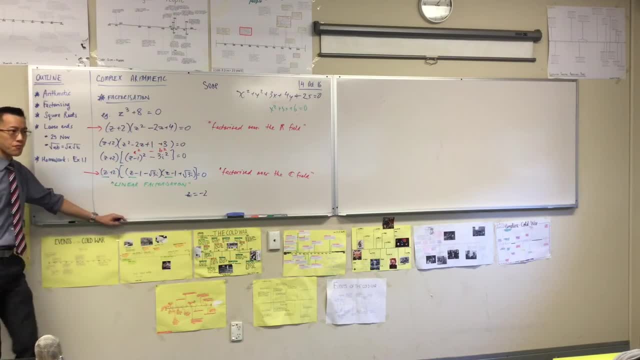 What are the other two solutions? Look carefully at this. So for this one I need 1 plus root 3i. to balance this out so that that becomes 0.. 1 plus root 3i, And have a look at this one. 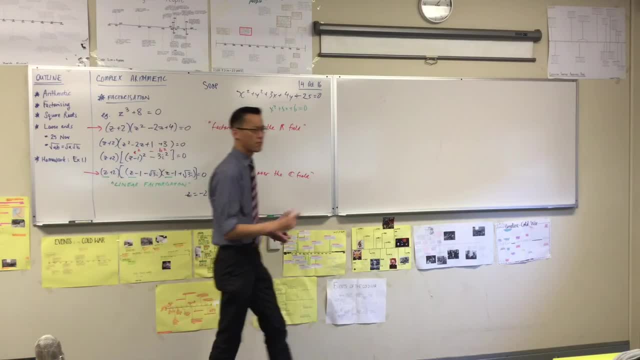 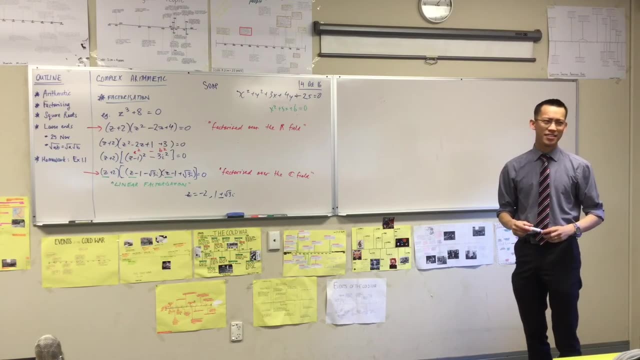 1 minus huh. What are those called? again, Complex conjugates. Is that a coincidence that we've got complex conjugates? There's never a coincidence in mathematics. Okay, we'll come back to that idea Now. hold on a second. 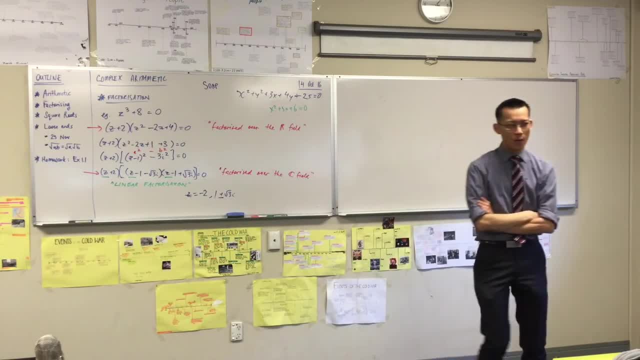 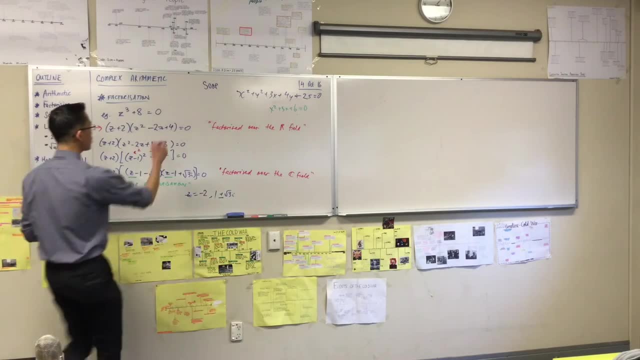 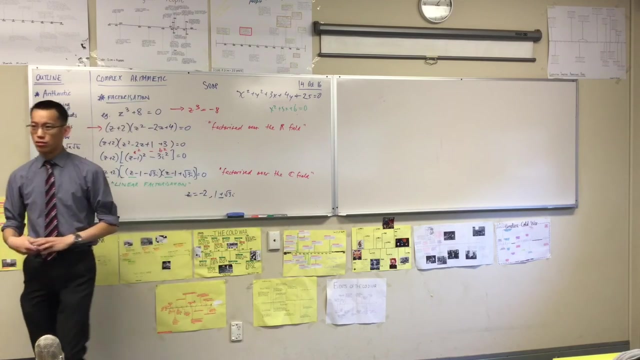 Hold the front door. What did we start with at the beginning of this question? z cubed plus 8 equals 0.. Now I can rewrite this right. I can just rewrite this as: z cubed equals minus 8.. Now if I gave that to you as a 2-unit student or as an extension, 1 student. 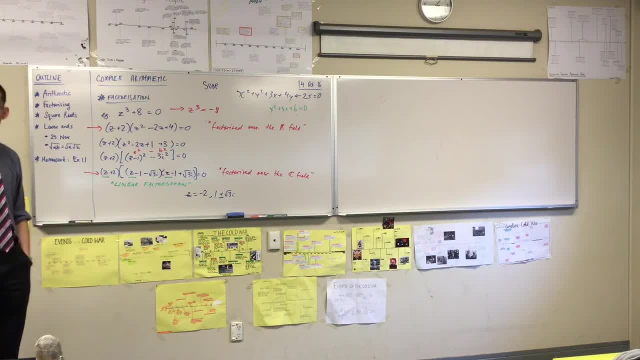 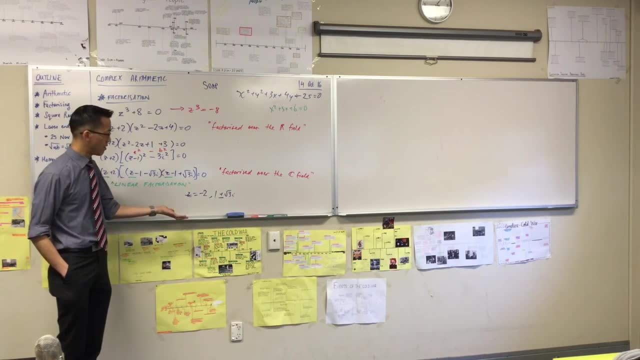 or even as like a year 8 student, you would have said: I know what the answer to that is. The answer is negative, 2. And that's the only answer, right? But now that you know there's more to the universe. 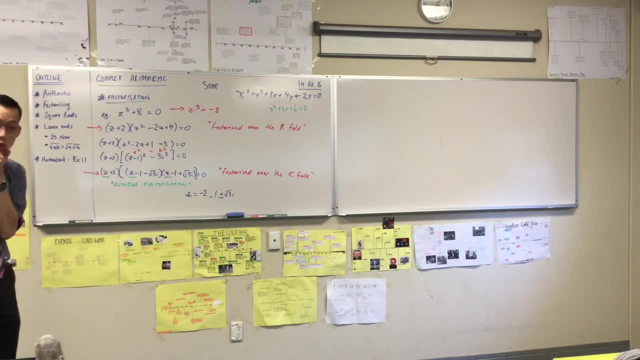 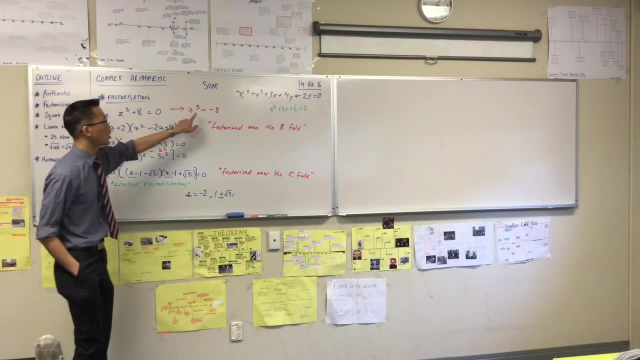 than just the real numbers you thought of before. Now you know, there aren't just. there isn't just one answer, There are three, which is exactly what you should expect, because you're taking the cube root right. Like you know, square roots. 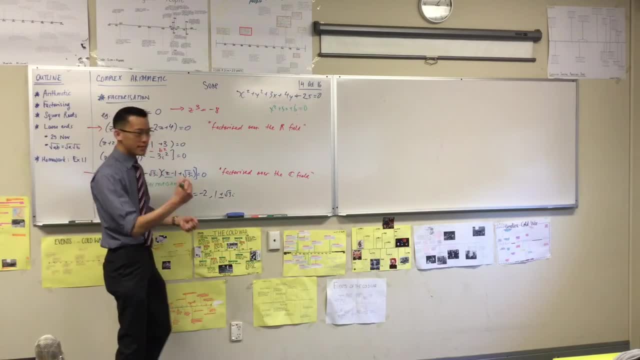 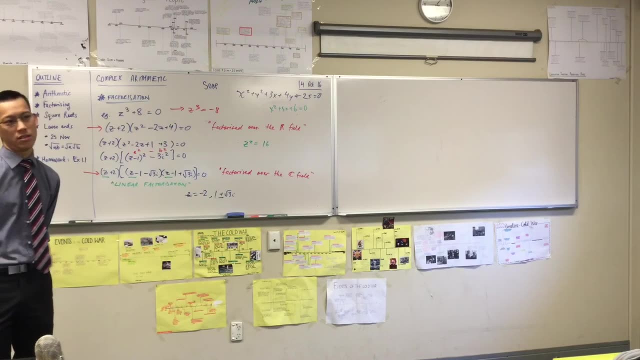 This is actually the next idea we're kind of segwaying into right. If I said to you: z squared equals 16, you know there are two answers. Everyone knows there are two answers, Even like little little kids know there are two answers, right. 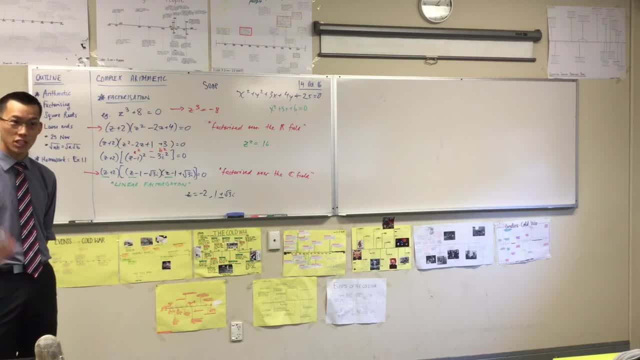 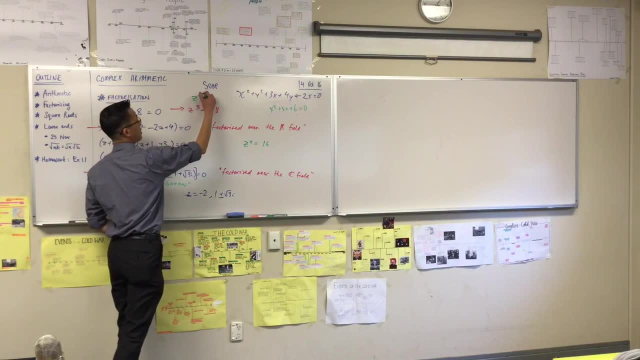 And if I said to you z to the 4,, z to the 5,, you should expect there's lots and lots of answers. This has three answers. In fact, z to the n equals anything always has n answers, right, Whether it's 2 or 3 or 50.